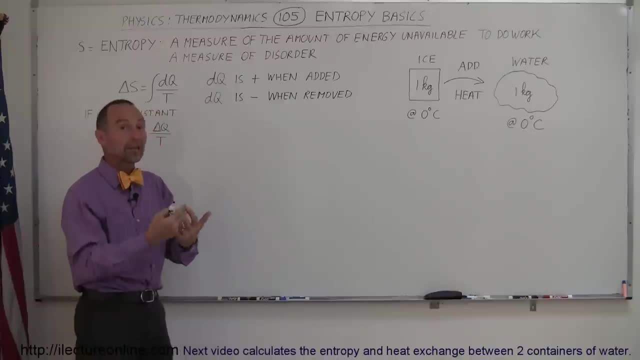 And throughout the universe. an exchange of energy usually results in an increase in the entropy. So what we usually try to do is measure or calculate that change in entropy. That little triangle there means change in. So we're looking for the change in the entropy. 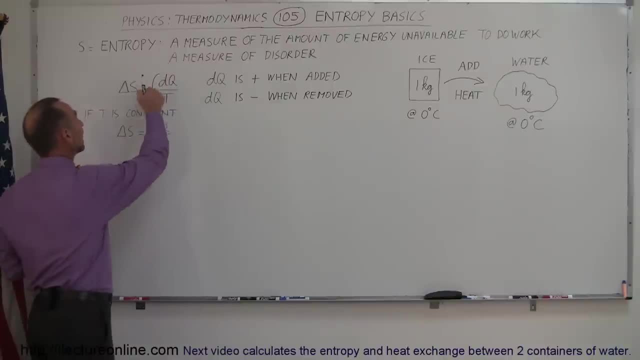 which is typically positive, and normally we calculate it by taking the integral of the exchange heat divided by the temperature at which that occurs. Now, typically in more simple problems, the temperature is kept constant, and so we can find the change in the entropy by simply calculating the difference in the temperature. 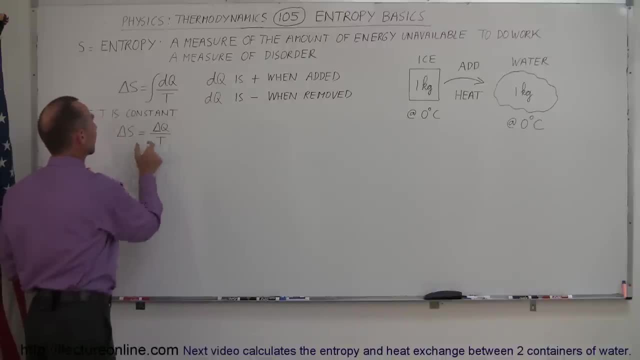 In the heat, or the amount of heat added to the object divided by the temperature of the object. Now be careful. DQ, which means the change in the heat, is positive when the heat is added to the object and DQ is negative when it's removed from the object. 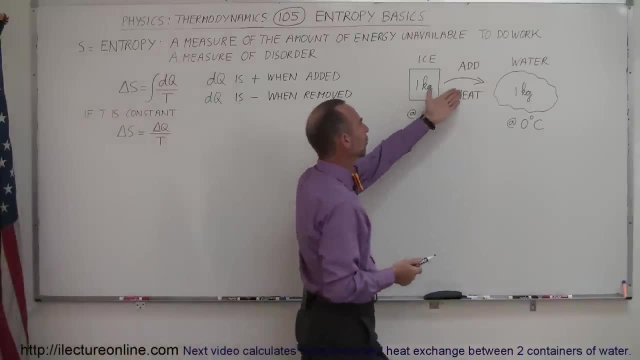 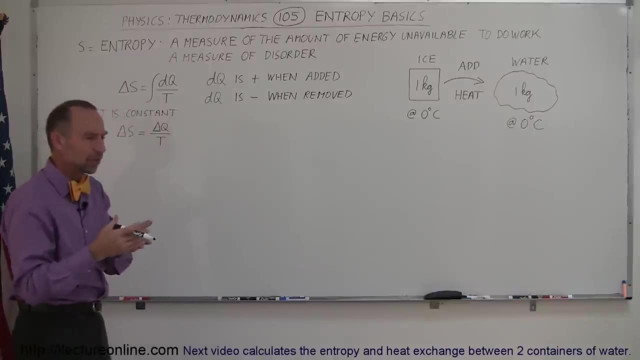 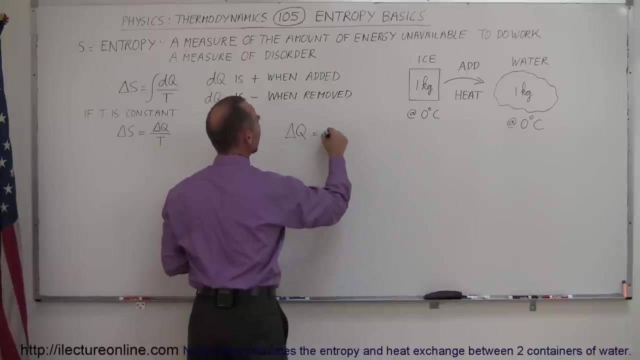 Alright, so let's do an example. Let's take the one kilogram of ice converting to water. Now, when we make ice melt, we have to add heat to it. and how much heat do we need? We need to add. well, that is the delta q. my pen started drying up here, so the delta Q is equal to. 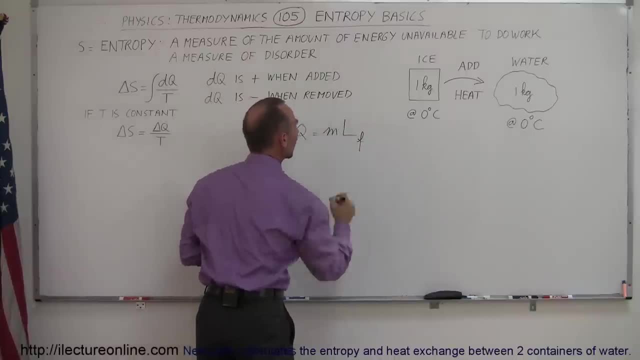 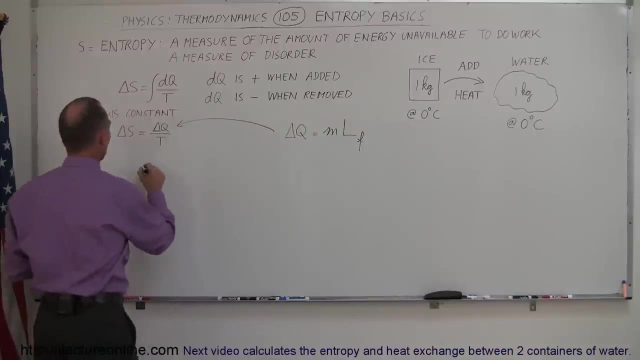 the mass of the ice times the latent heat of fusion of the ice. So that is the amount that we need to put in there and since we're adding heat to the ice, that quantity is positive. So this is going to be equal to the mass of the ice times the latent heat of fusion divided. 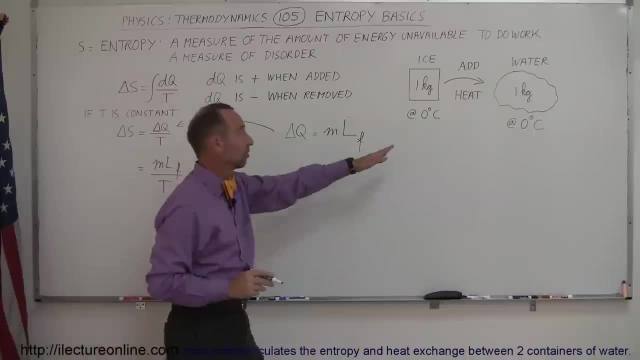 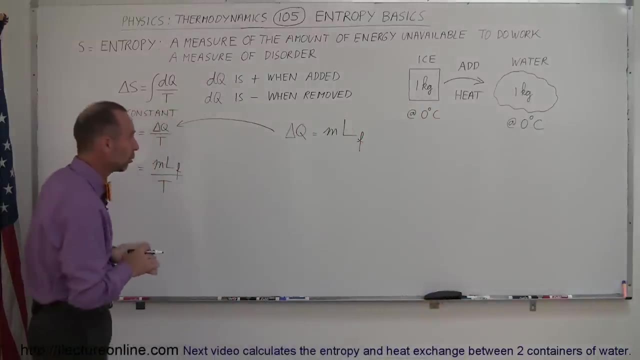 by the temperature which occurs. Now, of course, the ice is at zero degree centigrade. it doesn't change temperature when it turns into water, So the temperature that we're would be 0 degrees centigrade converted to Kelvin, which would be 273 Kelvin. 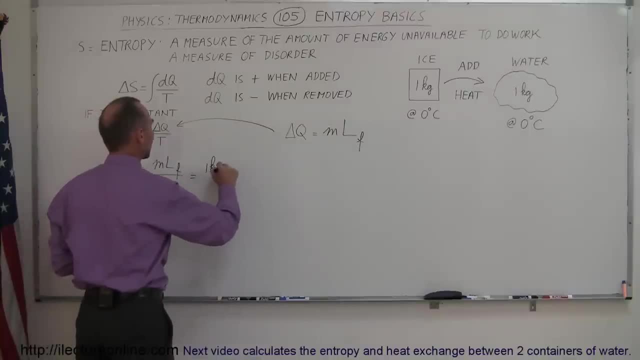 All right. so this would be 1 kilogram times the latent heat of fusion. Now that would be 4186 joules per kilogram. to change 1 kilogram of water 1 degrees centigrade. We multiply that times 80, which gives us the latent heat of fusion. 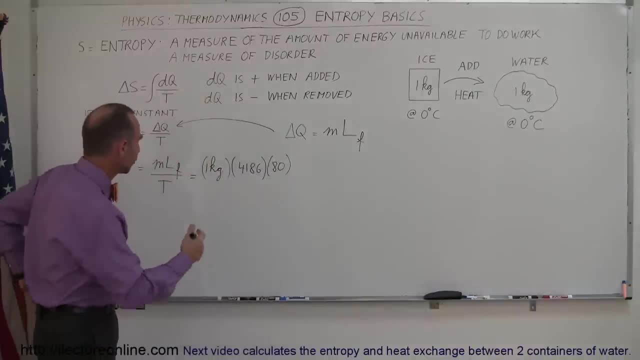 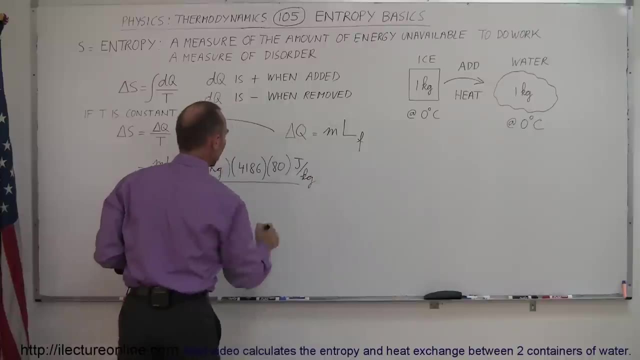 for ice, for going from ice to water, and then we divide that, and of course I need to. that would be joules per kilogram, and then we have to divide that by the temperature, which is 273 Kelvin. Now notice that the kilogram cancels out and.